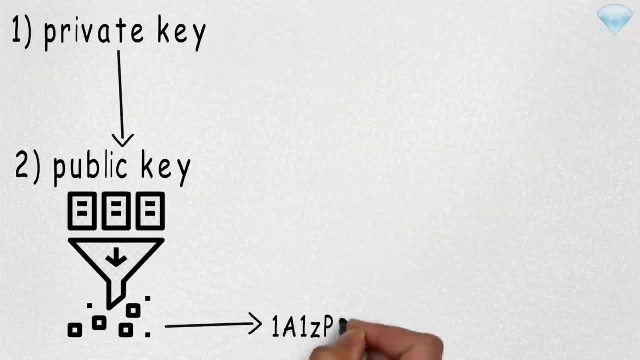 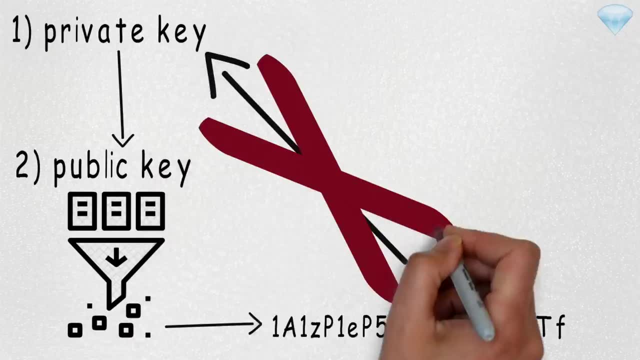 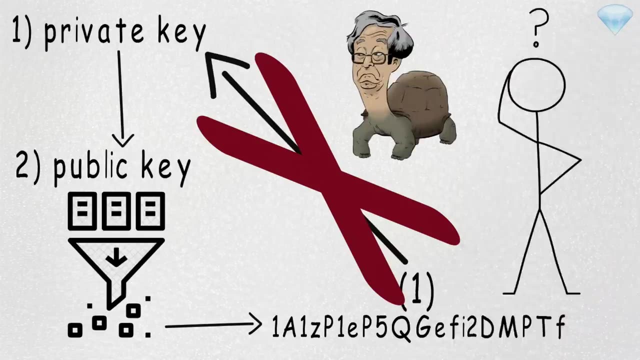 by hashing that public key you got your address. Hopefully you cannot choose the address first and then determine the private key from that. Otherwise you could determine the private key for any address using this method. Wait, what? What is Satoshi's address again? 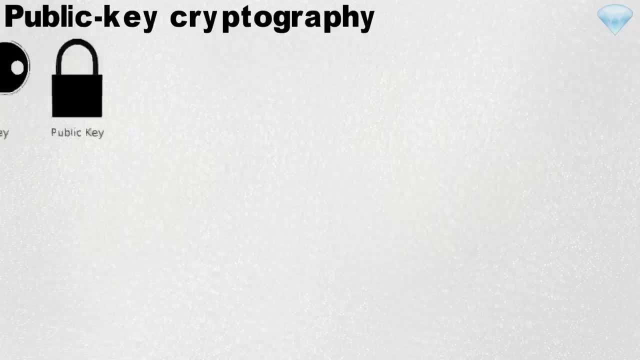 Public Key Cryptography. Public keys, private keys and digital signatures are from the basic components of the public key cryptography. No matter what mathematical basis is used to implement public key cryptography system, it must satisfy the following: 1. It is computationally impossible to 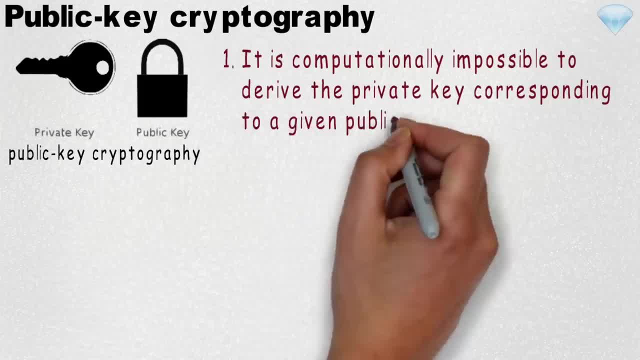 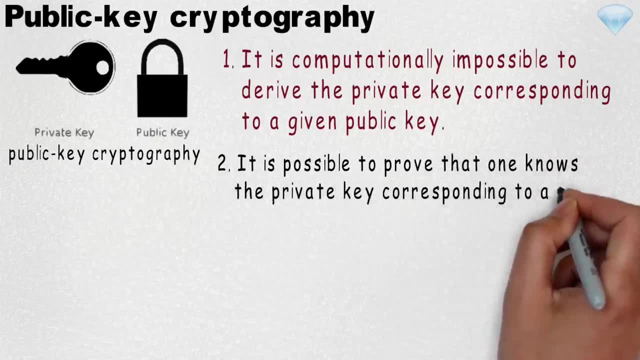 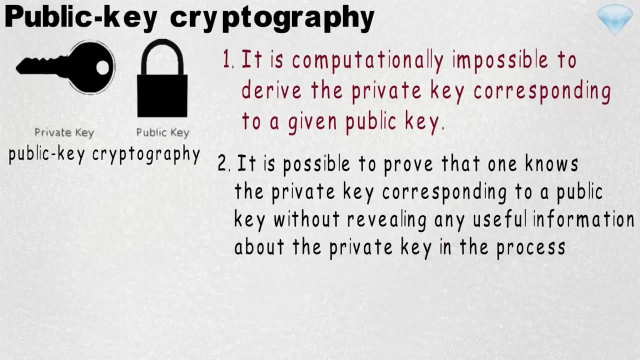 derive the private key corresponding to the given public key. 2. It is possible to prove that one knows the private key corresponding to the public key without revealing any useful information about the private key in the process? 1. One way to do a public key cryptography is with elliptic curves. Another way is with RSA. 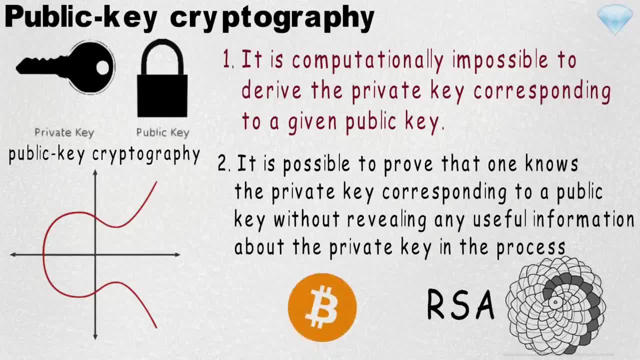 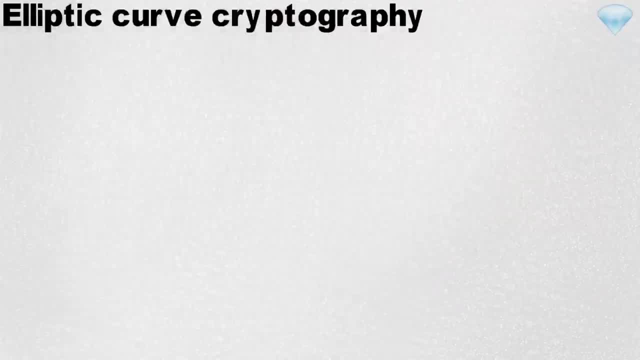 which revolves around prime numbers 2.. Most cryptocurrencies, like Bitcoin and Ethereum, use elliptic curves, Elliptic Curve, Cryptography. Now the question is: what is an elliptic curve? An elliptic curve contains all of the following points that satisfy an equation of the following form: y² equals x³ plus ax plus b. 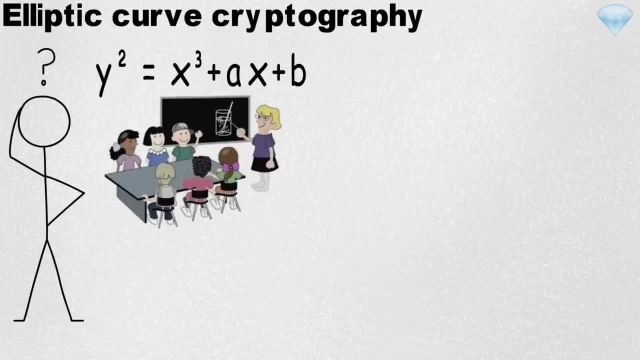 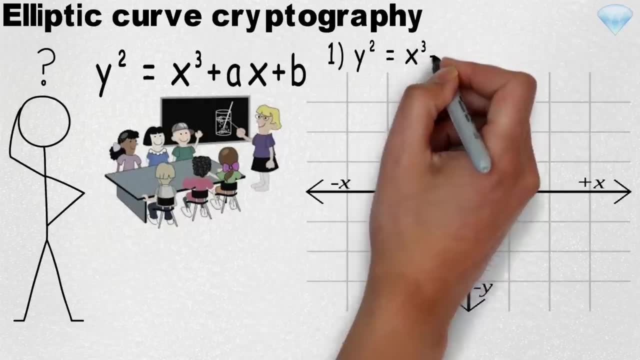 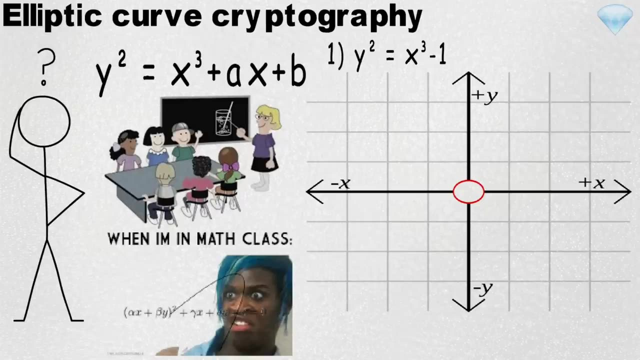 Let's go back- I don't know, 8th grade or whatever- and look at some of the functions of elliptic curves: 1.. First example is: y2 equals x³ minus 1.. If you're, math sucks and you did not pay any attention in your geometry class, 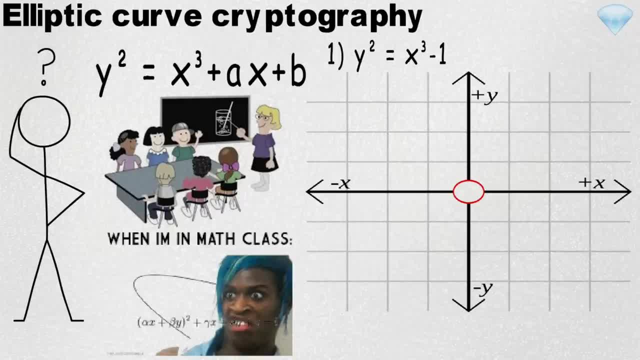 here's how we can draw this function. We have x-axis and y-axis And we have an equation. Now we are going to plug random integers into x variable to find y 2. If x equal one, then x³ also one. 5. Right now there's even more available factor ways toath game of Lyft's exam and, of course, this advantages that you may do in class. So please ask if you like this math application 464. tried to fix it, but this will help students keep learning alphabets. 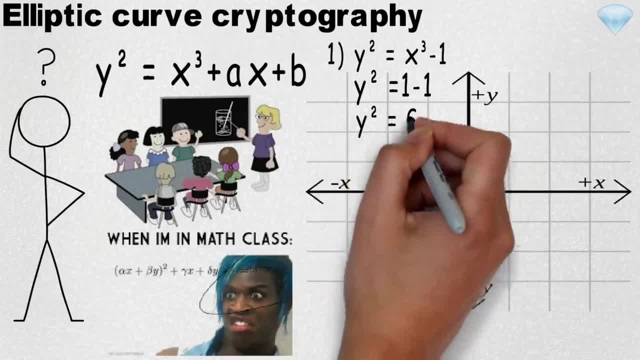 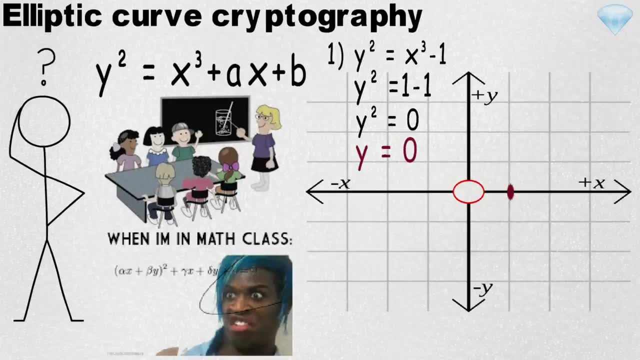 minus 1 equals 0. Then y squared equals 0. Therefore y equals 0.. So when x equals 1, then y equals 0 respectively. Now let's say x equals 3. Then 3 cube is 27.. 27 minus 1 is 26.. 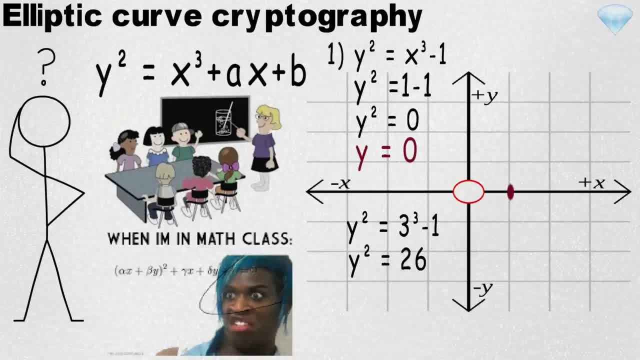 Then y squared equals 26.. Therefore y equals plus minus square root of 26 and it equals to approximately plus minus 5.01.. So when x equals 3, then y equals plus minus 5.01 respectively. Now we can plot those numbers. Of course it would be much better to give more integers to x. 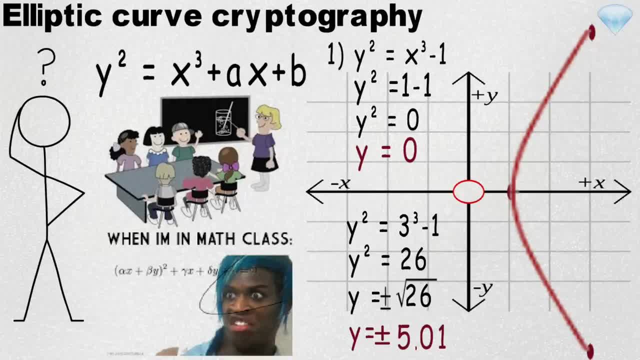 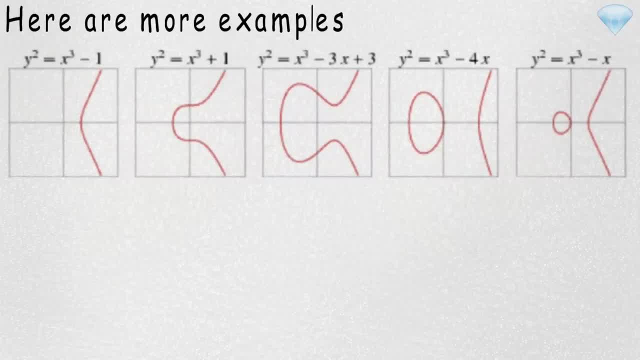 but we do not have a lot of time. Well, you got the idea. Here are some examples of elliptic curves. Notice: all elliptic curves are symmetrical about x. The elliptic curve used by Bitcoin, Ethereum and many other cryptocurrencies is called: 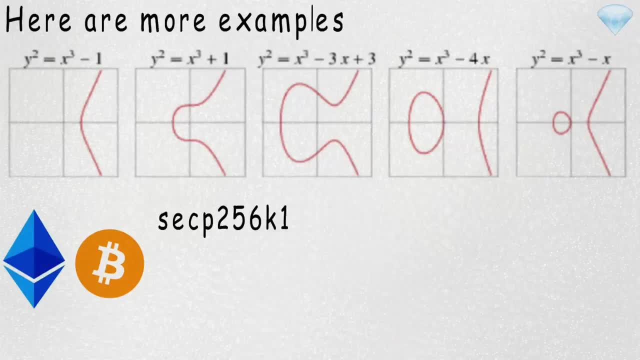 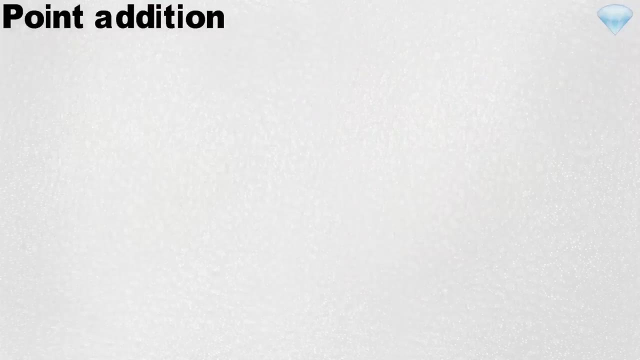 SACP256K1.. The equation for the SACP256K1 curve is: y squared equals x cubed plus 7.. This curve looks like this Point addition: You know how you can add two numbers together to get the third one. Well. you can do that by adding two numbers together. So you can add two numbers together to get the third one. Well, you can do that by adding two numbers together to get the third one. Therefore, you will not need special numbers. What is 1968.? 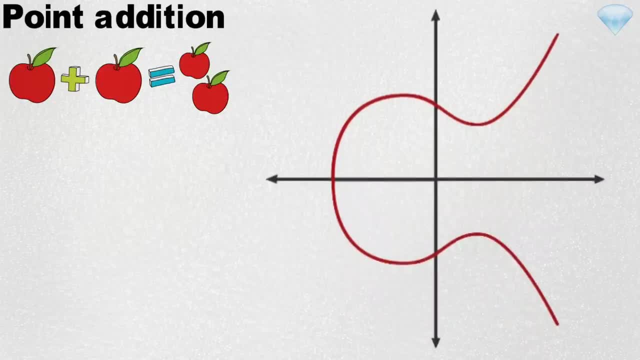 The first number, which you do not need, is across the cross. This one is again on the second line. Then you can subtract 2 points together To add two points on an elliptic curve. you first find the line that goes through those two points. 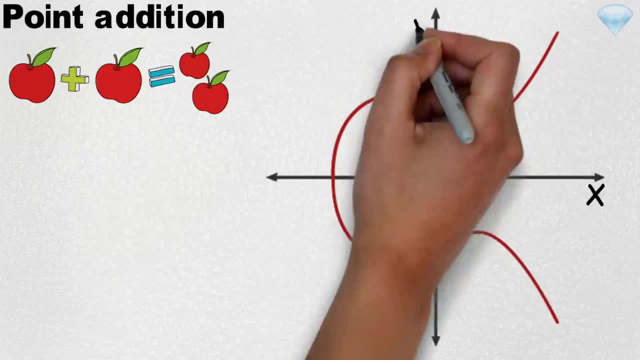 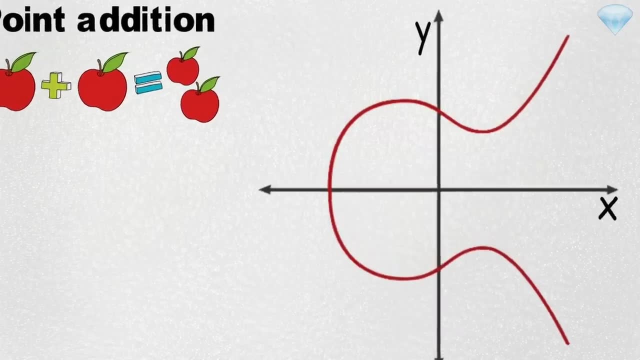 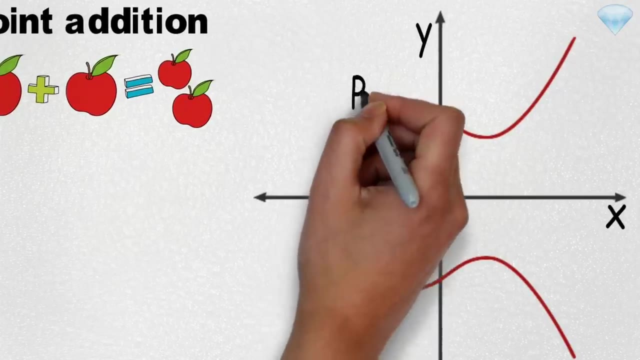 Then you determine where the line intersects the curve at the third point. Then you reflect the third point across the X-axis and whatever point you get from that is the result of adding the first two points together. For example, let's say you want to add the following two points together: 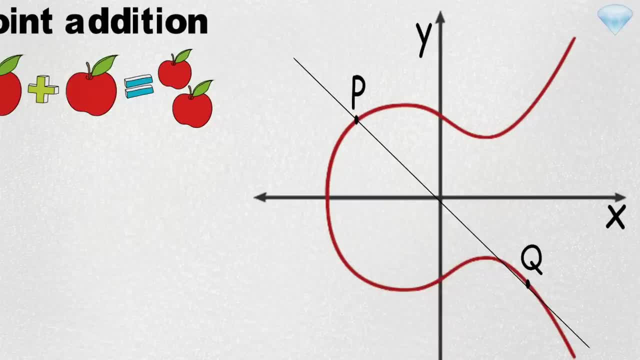 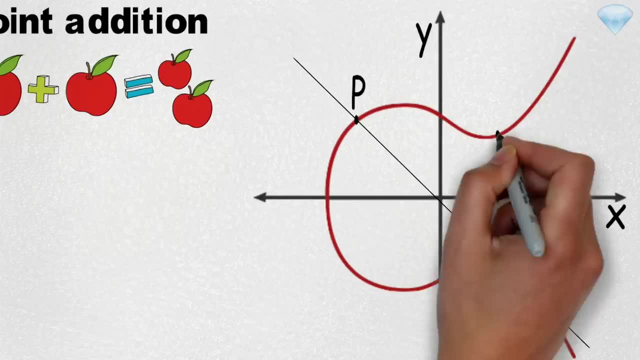 First you find the line that goes through those two points. Then you find the third point on the curve that line intersects. Then you reflect the point across the x-axis. let's call it R. Therefore P plus Q equals R. 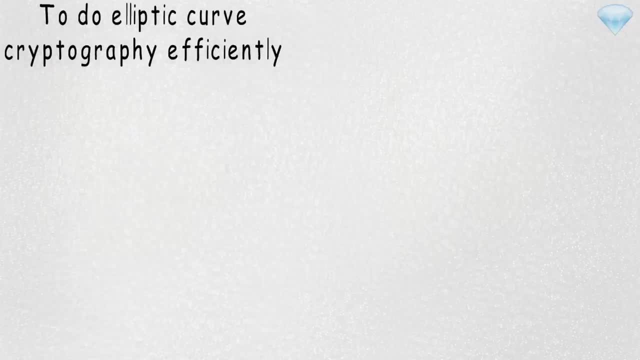 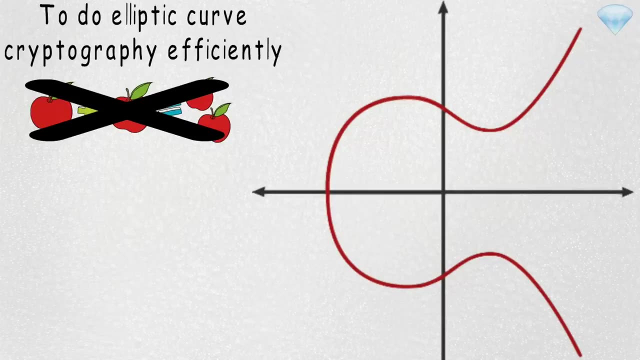 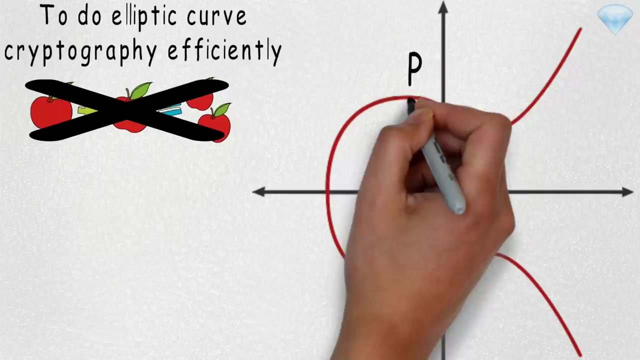 To do elliptic curve cryptography efficiently, rather than adding two arbitrary points together, we specify a base point on the curve and only add the point to itself. For example, let's say we have the following curve: with the base point P, Initially we have P or 1 multiplied by P. 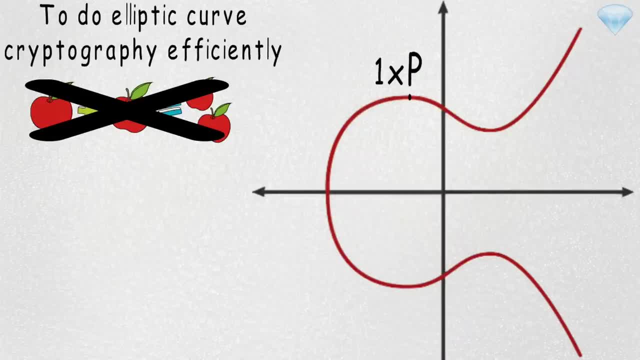 Now let's add P to itself. First we have to find the equation of the line that goes through P. There are infinite such lines. In this specific case, we use tangent line. If you do not know what tangent line means, here is the definition. 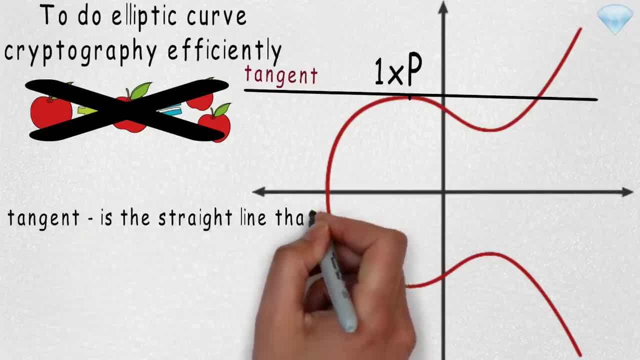 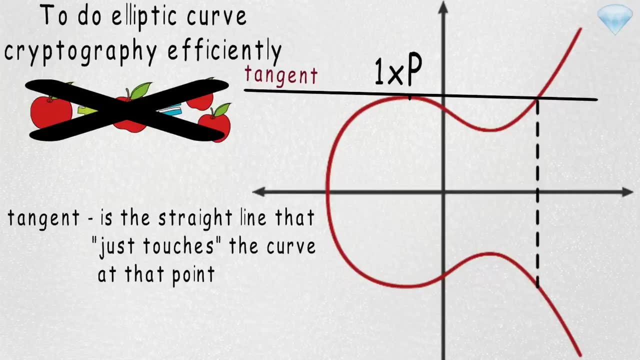 The tangent line to a plane curve at the given point is a straight line that just touches the curve at that point. Now we find the third point: that this line intersects and reflected across x-axis. Therefore P adds to itself, or P plus P equals 2P. 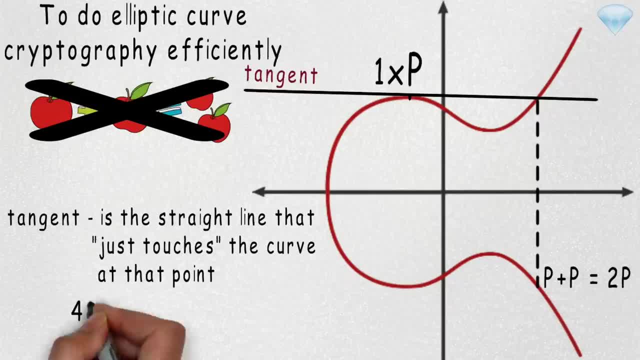 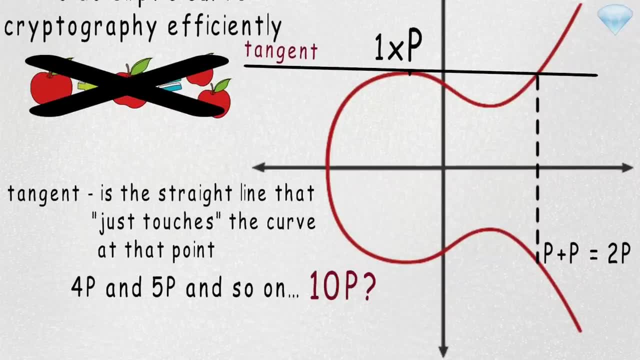 We can continue to add P to itself, to compute 4P And 5P and so on, But how many steps would it take to compute 10P? It would appear to take 9 steps, Because 10 multiplied by P is P adds to itself 10 times. 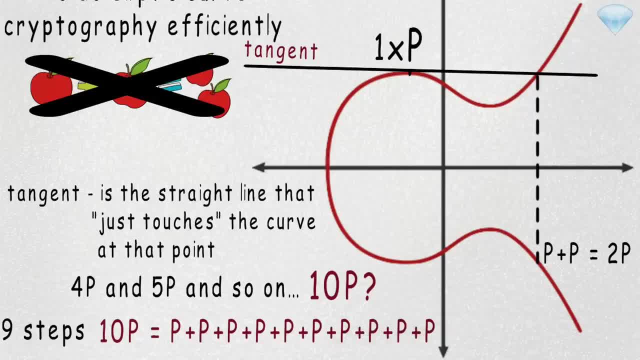 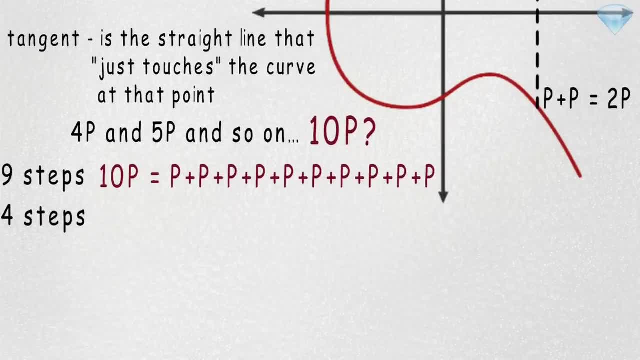 Which requires 9 points addition operations. It turns out that we can compute 10 multiplied by P in just 4 steps. This is because the following property holds 4 points addition. We can take out P and we get n plus r in parentheses, multiplied by P. 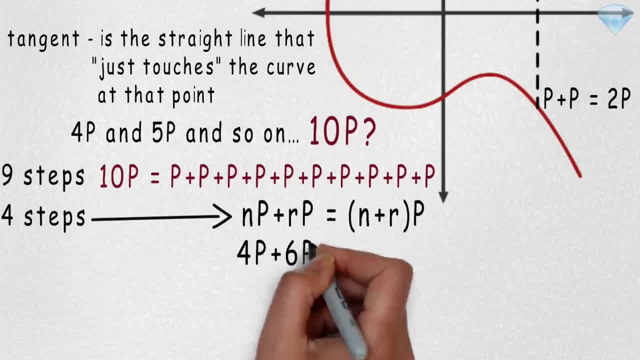 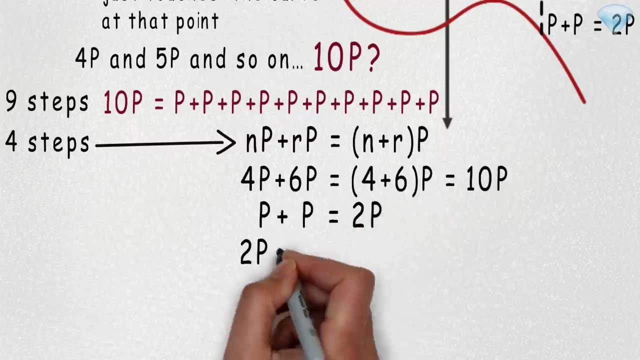 For example, 4P plus 6P equals 4 plus 6, in parentheses, multiplied by P equals to 10P. Therefore, the first way to calculate 10P is as follows: P plus P equals 2P. 2P plus 2P equals 4P. 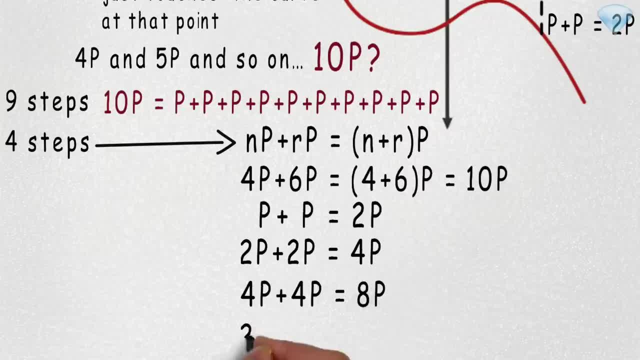 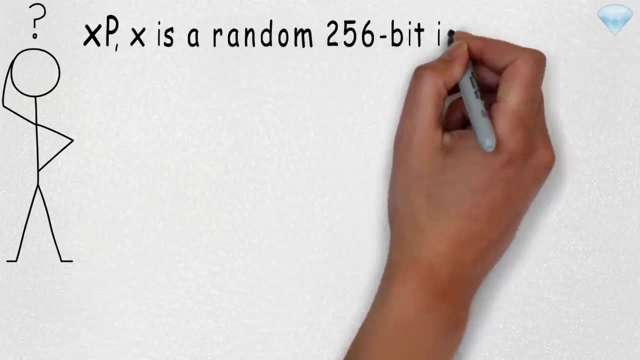 4P plus 4P equals 8P. 2P plus 8P equals 10P, which only requires 4 points addition operations. How many steps would it take to compute XP where X is a random 256-bit integer? 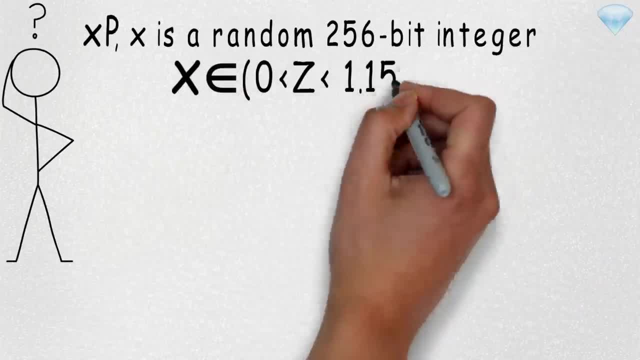 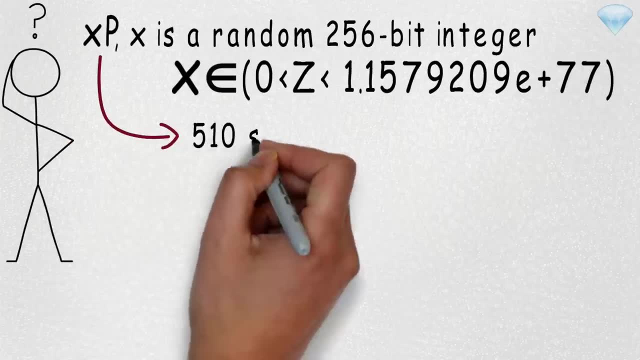 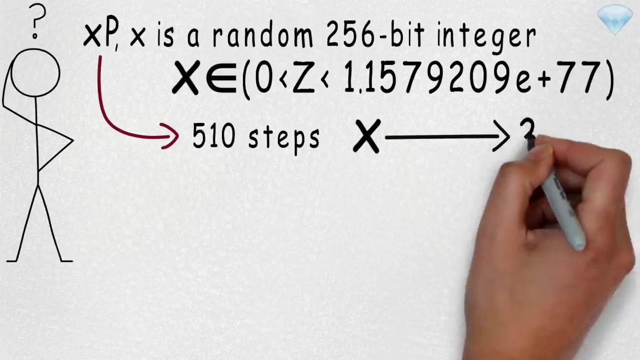 In this case X can range anywhere from 0 to a very large integer. It turns out that computing XP would never require more than 510P point addition operations. I'm just going to give you fast explanation why. At most the binary expansion of X will contain 256 elements, that is, up to 2 to the power. 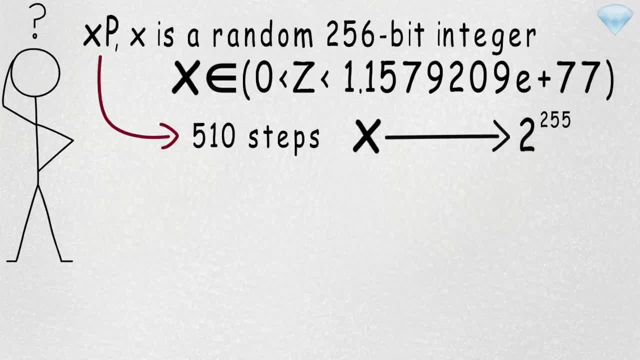 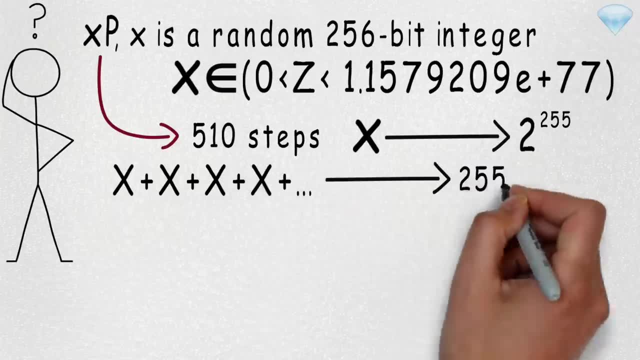 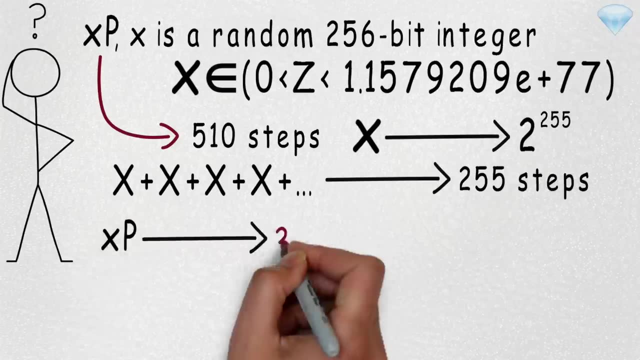 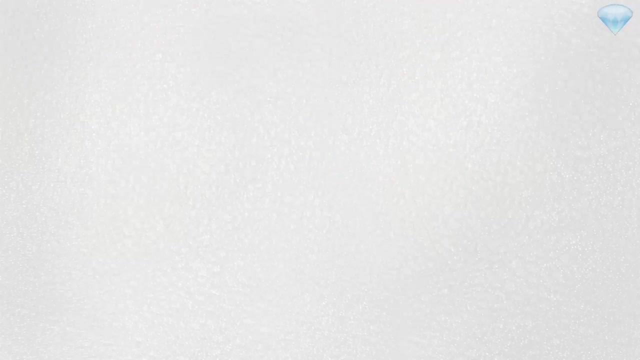 255.. So we won't ever have to add more than 256 points together. Therefore, the second step will require at most 255 points addition operations. Therefore, computing X times P will take at most 255 plus 255 equals 510 points addition operations. 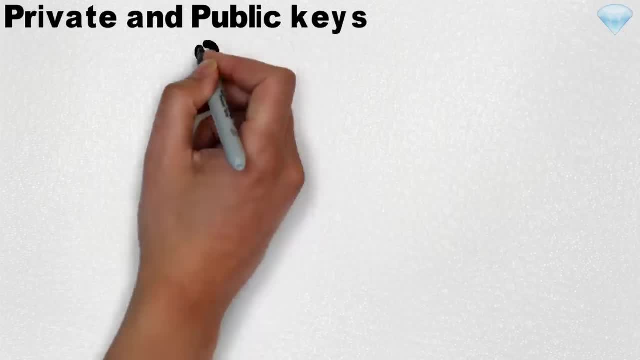 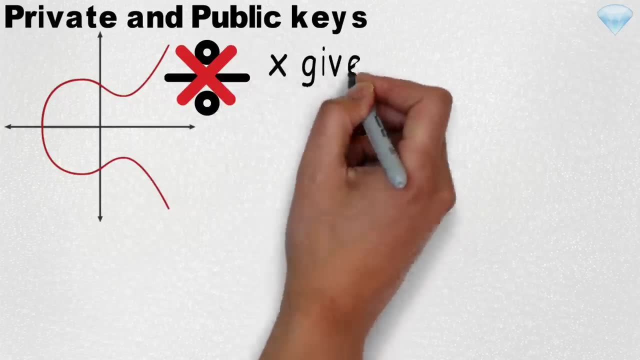 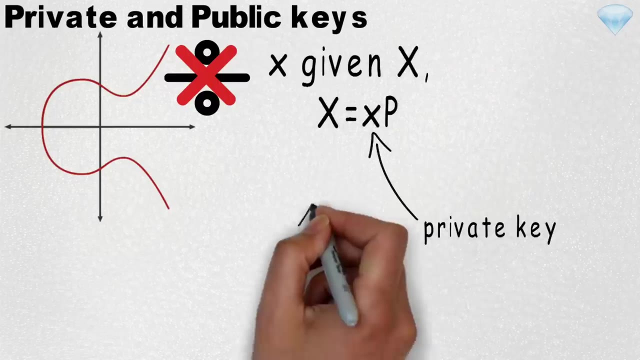 Private and public keys, Since the division does not exist in elliptic curve cryptography. therefore, you cannot figure out small X given large X where X equals 2.. It might be convenient to make small X your private key and large X your public key Your. 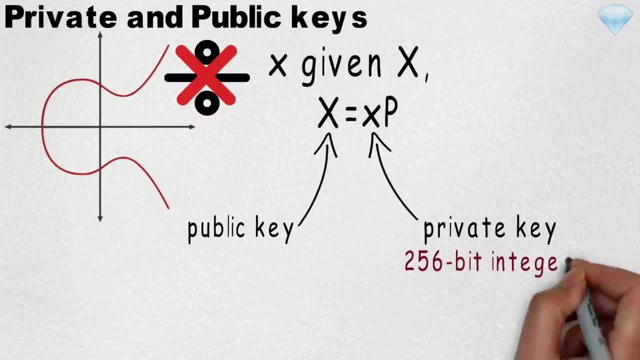 private key would then be random 256-bit integer and your public key would then be X and Y coordinates of the point on elliptic curve. This would satisfy the following property of private and public keys: It is computationally impossible to derive the private key corresponding. 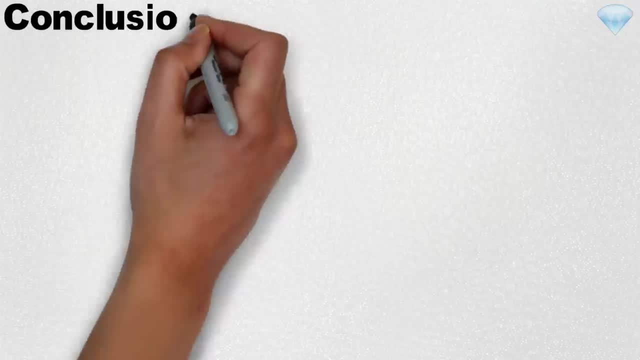 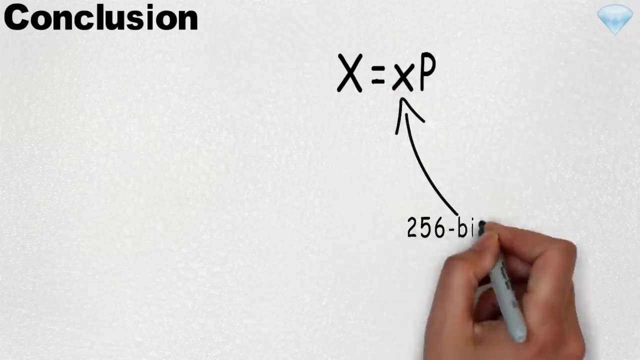 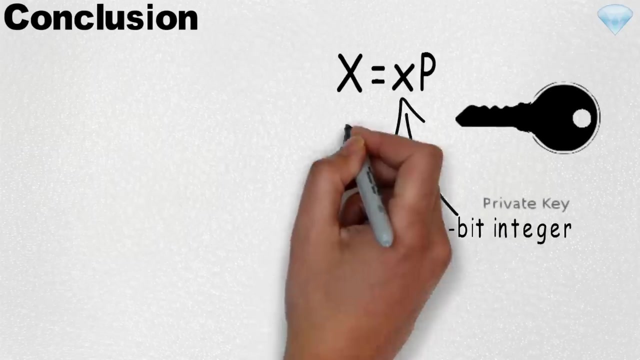 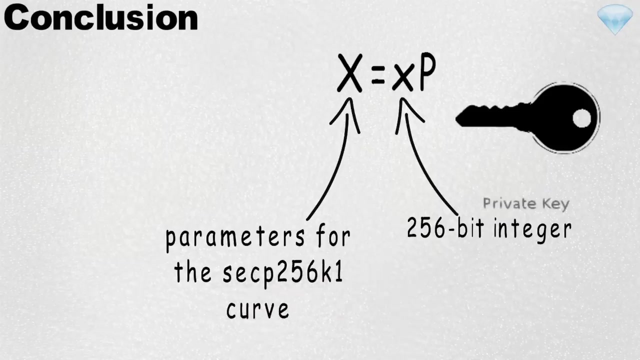 to a given public key. Conclusion: If you want to obtain Bitcoin address or Ethereum address, you generate random 256-bit integer small X. Small X is then your private key. Then you compute: large X equals small X times P using a parameter for the secp256k1 curve. Large X will be your public key, Your public. 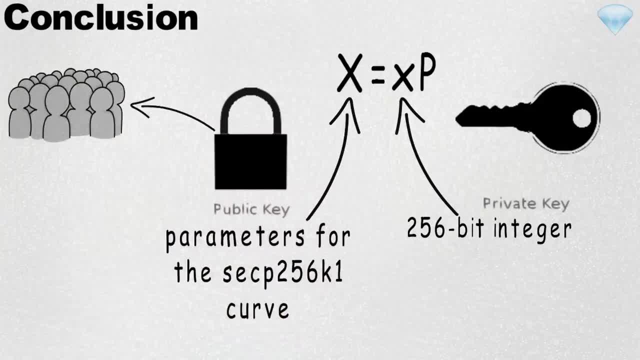 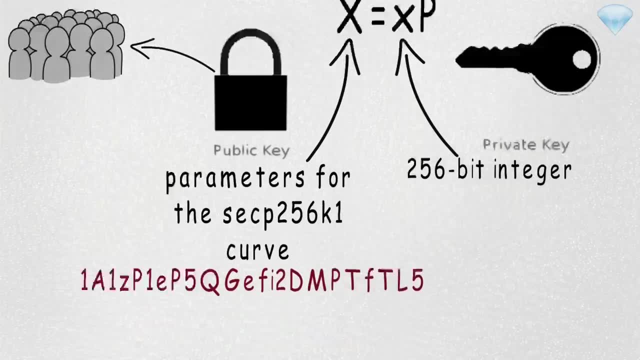 key is safe to give out and cannot be used to determine your private key. So you can use your private key. If you hash your public key, you will obtain your address. So this is the end. Let me know what do you guys think about the math behind elliptic? 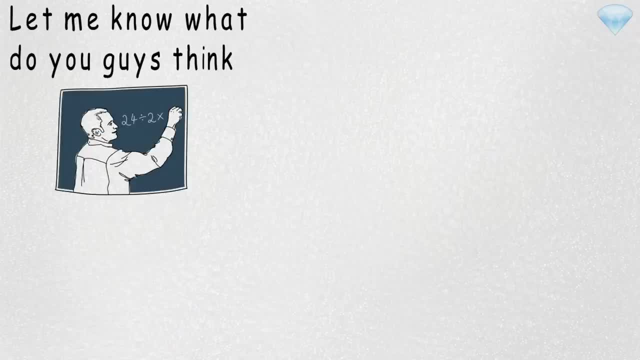 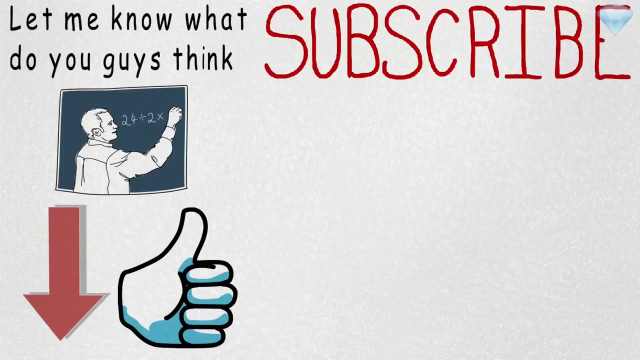 curve cryptography. Is it too complicated or not? Leave your thoughts in the comment section below. If you enjoyed this video, hit that like button, And if you are new to this channel, do not forget to subscribe for more animated videos about cryptocurrency and blockchain technology. Other than that, thank you for watching and see you next time.